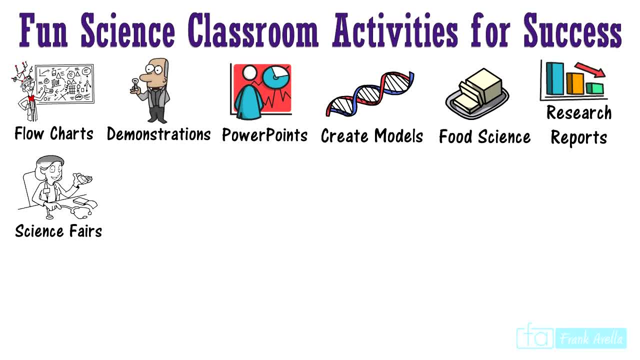 put it on a trifold board. You'll need to get the principal on board, but why wouldn't they? Early students can come down in the afternoon and view their work. When an active student makes progress, an active student can take a course or a class. 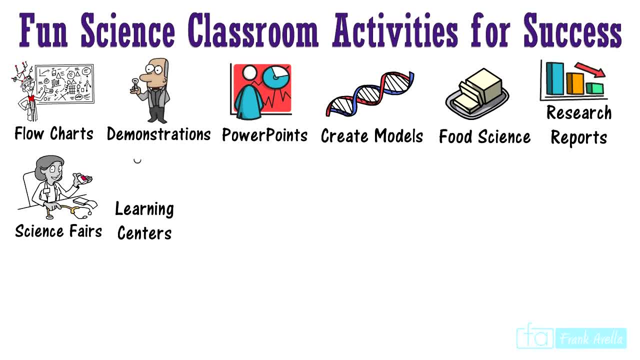 Learning centers are a classroom activity where several different assignments are located at tables. in the classroom, Students rotate as a group from table to table. Marzano's research shows that one of the best ways to learn new information is to compare and contrast to other known information. As an activity, have students complete a Venn diagram. 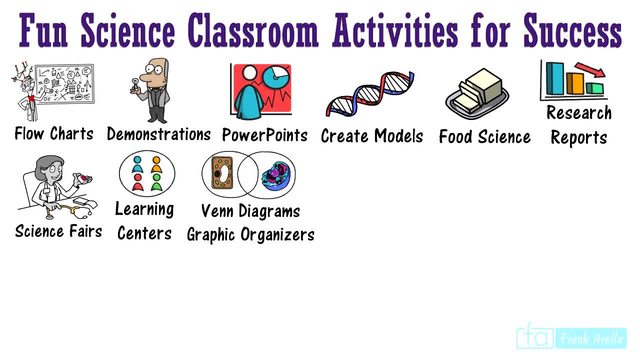 or any other type of graphic organizer. When I was in school, we were allowed to perform dissections. Today, schools with a computer can do that and may take questions. Even some are going to have to ask students if they can answer questions. 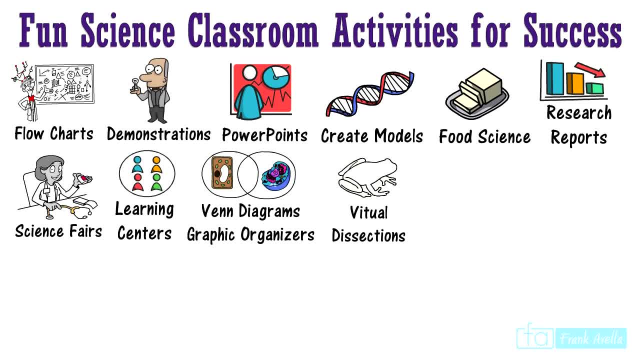 limited resources, use virtual dissection. You can find them online and it's much easier than having to do all the work of setting up and cleaning after the real dissection. Games are always fun if the teacher makes it that way. Try a science bingo or a science jeopardy. You'll need 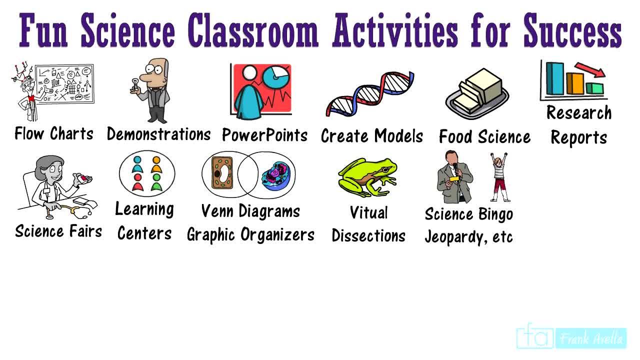 to give a prize. if you want maximum engagement, Maybe a small bag of chips. Poster boards were always a staple of my classroom teaching. Students can create posters on the world of biomes. They can do the tundra, the desert, deciduous forests, and then they present that information. 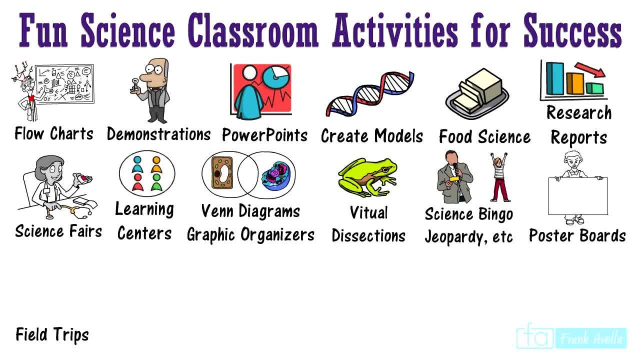 to the classroom. I've always been a big advocate for field trips. It provides an opportunity for students to make a connection between the content and real life. It also gets the students out of the boring classroom. Classroom debates may seem like an activity meant for social studies classes. 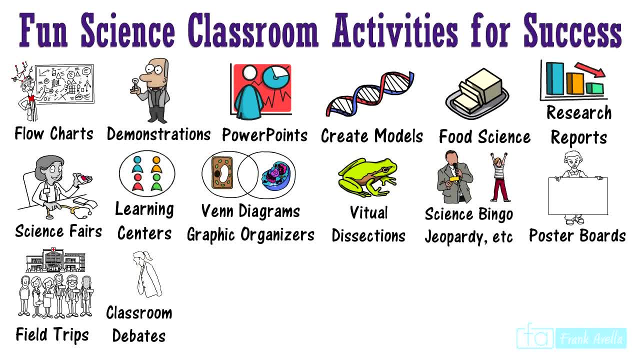 but it doesn't have to be. Allow students to debate the effects of global warming. Students make arguments and support their arguments with scientific evidence. Lab experiments are requirements for several secondary science courses. At the end of the day, performing lab experiments is an essential function of science. Mr Zellman has his environmental 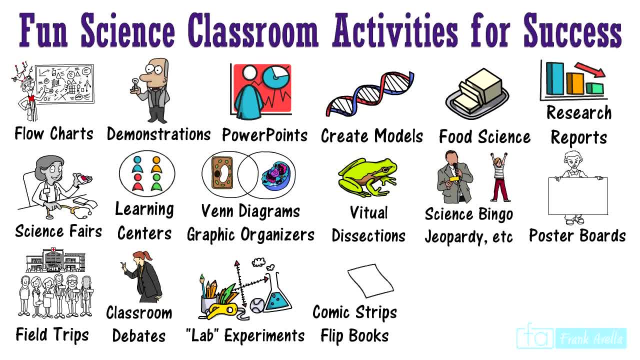 science, students create comic strips on environmental issues such as oil shortage and electric cars. For biology, he has students create a flipbook for mitosis and meiosis. Another activity is to do current events in science class. Students can read web articles on the daily news in the scientific community.